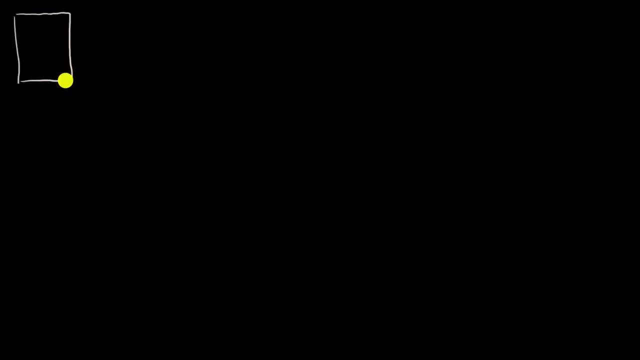 Let's say that I run a website that currently has this off-white color for its background, and I know the mean amount of time that people spend on my website- Let's say it is 20 minutes- and I'm interested in making a change. 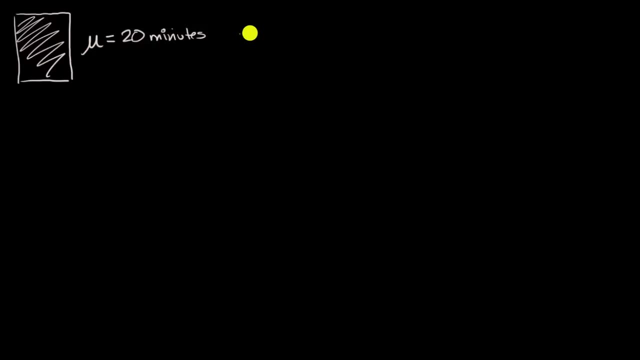 that will make people spend more time on my website. My idea is to make the background color of my website yellow, But after making that change, how do I feel good about this actually having the intended consequence? Well, that's where significance tests come into play. 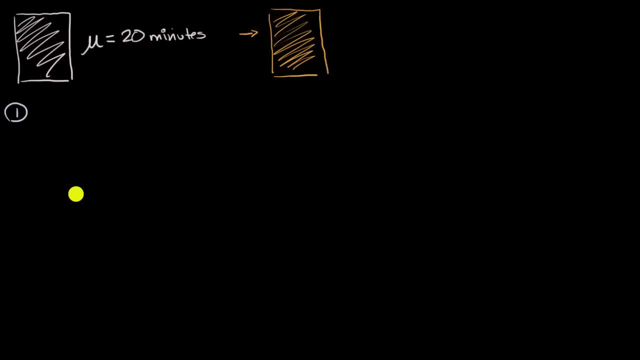 What I would do is first set up some hypotheses: a null hypothesis and an alternative hypothesis. The null hypothesis tends to be a statement that hey, your change actually had no effect. There's no news here, And so this would be that your mean. 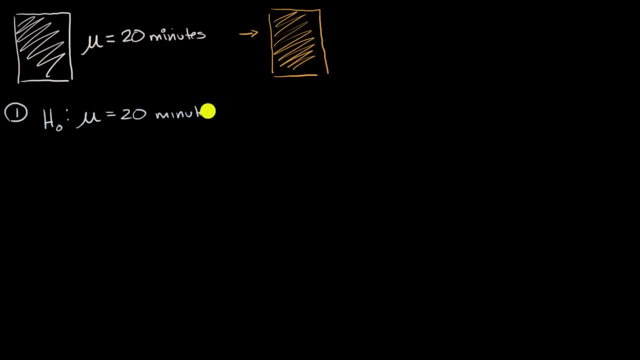 is still equal to 20 minutes is still equal to 20 minutes after, after the change to yellow in this case, for our background, And we would also have an alternative hypothesis. Our alternative hypothesis is actually that our mean is now greater because of the change. 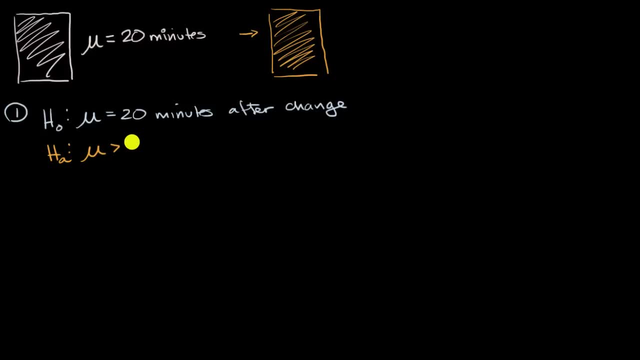 that people are spending more time on my site, So our mean is greater than 20 minutes after after the change. Now the next thing we do is we set up a threshold, known as the significance level, and you will see how this comes into play in a second 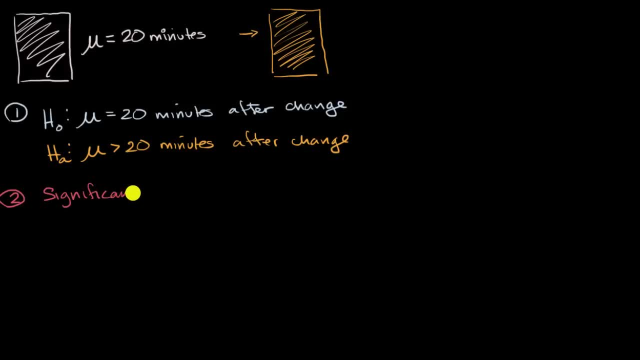 So your significance level. significance level is usually denoted by the Greek letter alpha, and you tend to see significant levels like 1 100th or 5 100ths or 1 10th or 1%, 5% or 10%. 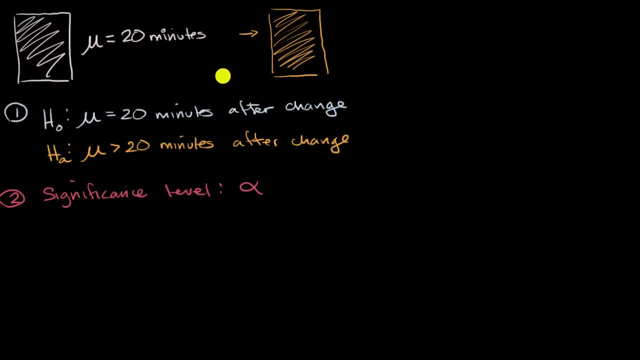 You might see other ones, but we're gonna set a significance level for this particular case. Let's just say it's going to be 0.05.. And what we're going to now do is we're going to take a sample of people visiting our site. people visiting our site. 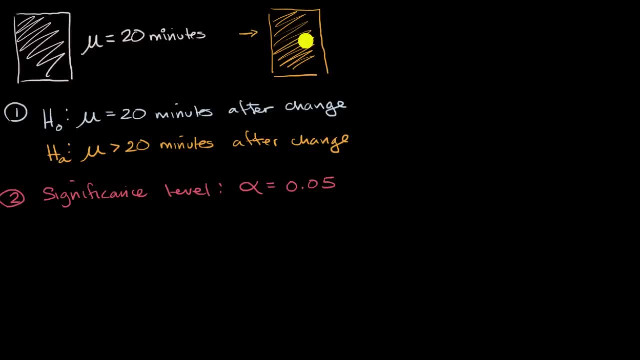 people visiting this new yellow background website and we're gonna calculate statistics, the sample mean, the sample standard deviation, and we're gonna say, hey, if we assume that the null hypothesis is true, what is the probability of getting a sample with the statistics that we get? 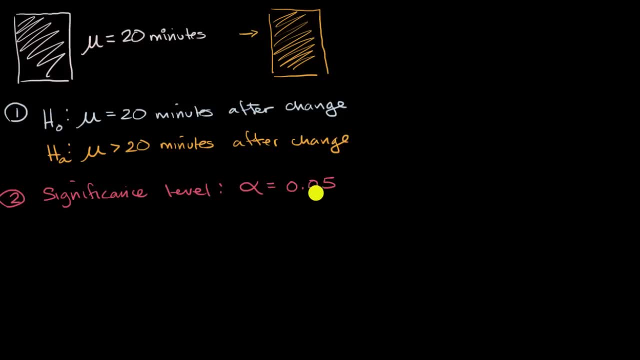 And if that probability is lower than our significance level, if that probability is less than 5 100ths, if it's less than 5%, then we reject the null hypothesis and say that we have evidence that it's true. We reject the null hypothesis and say that we have evidence. 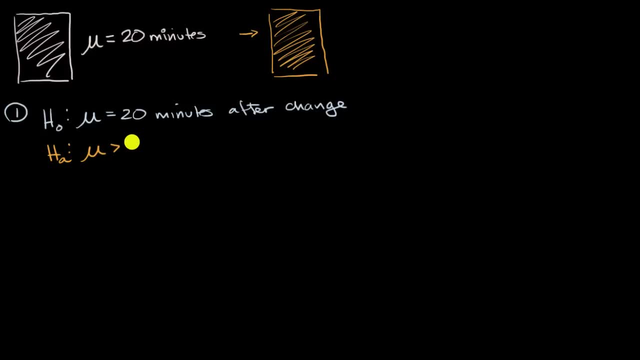 that people are spending more time on my site, So our mean is greater than 20 minutes after after the change. Now the next thing we do is we set up a threshold, known as the significance level, and you will see how this comes into play in a second 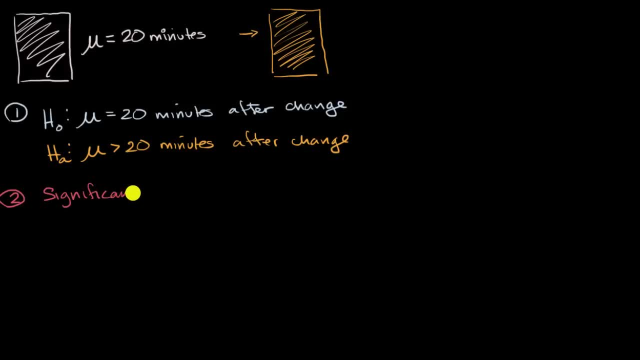 So your significance level. significance level is usually denoted by the Greek letter alpha, and you tend to see significant levels like one one-hundredth or five one-hundredths or one-tenth or 1%, 5% or 10%. 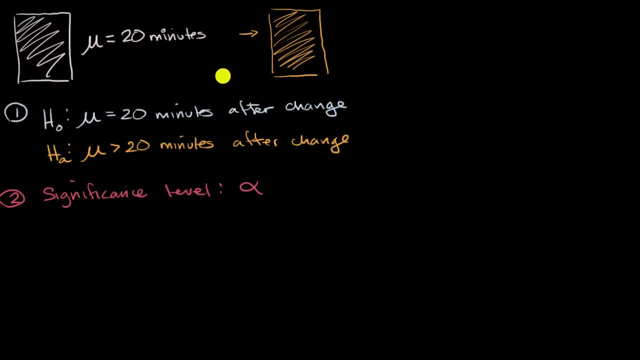 You might see other ones, but we're gonna set a significance level for this particular case. Let's just say it's going to be 0.05.. And what we're going to now do is we're going to take a sample of people. 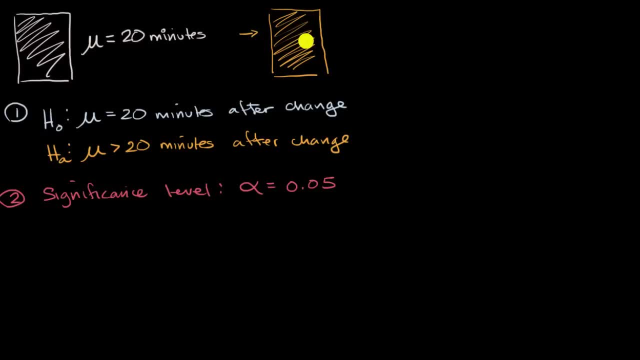 visiting this new yellow background website and we're going to calculate statistics, the sample mean, the sample standard deviation, and we're going to say, hey, if we assume that the null hypothesis is true, what is the probability of getting a sample? 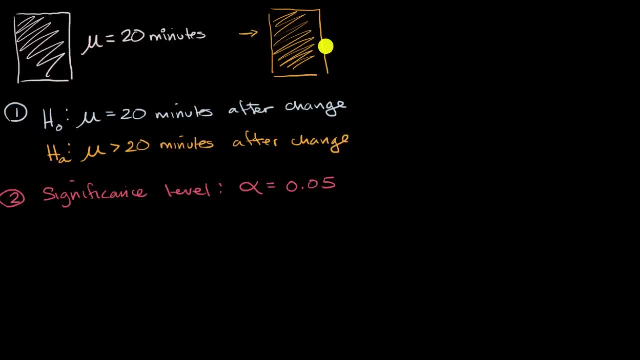 with the statistics that we get, And if that probability is lower than our significance level, if that probability is less than five hundredths, if it's less than 5%, then we reject the null hypothesis and say that we have evidence. we have evidence for the alternative. 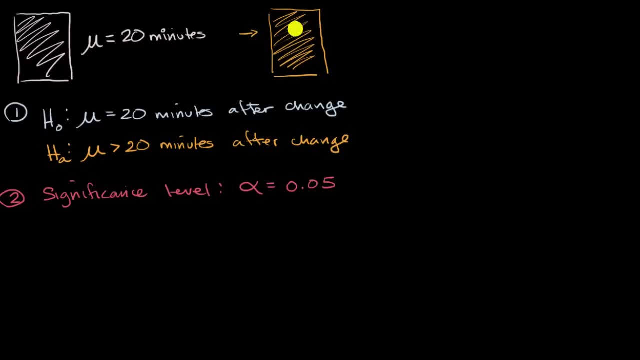 However, if the probability of getting the statistics for that sample are at the significance level or higher, then we say, hey, we can't reject the null hypothesis and we aren't able to have evidence for the alternative. So what we would then do? 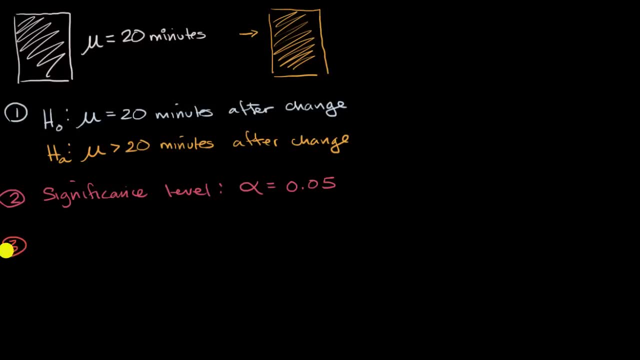 I will call this step three. In step three we would take a sample, Take sample. So let's say we take a sample size, let's say we take a hundred folks visit the new website, the yellow background website, and we measure sample statistics. 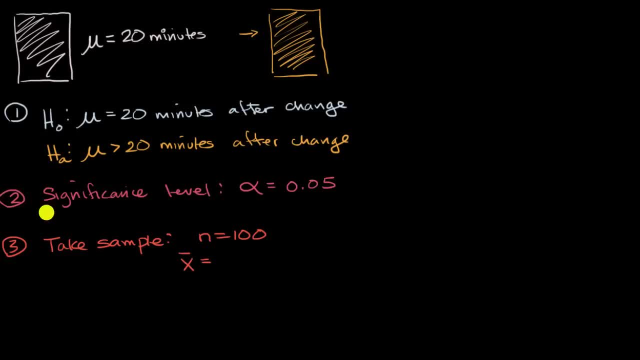 We measure the sample mean here. Let's say that the for that sample, the mean is 25, 25 minutes. We are also likely to if we don't know what the actual population standard deviation is, which we typically don't know. 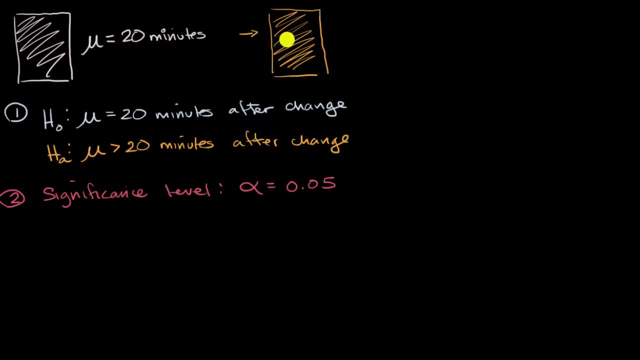 for the alternative. However, if the probability of getting the statistics for that sample are at the significance level or higher, then we say, hey, we can't reject the null hypothesis and we aren't able to have evidence for the alternative. So what we would then do? I will call this step three. 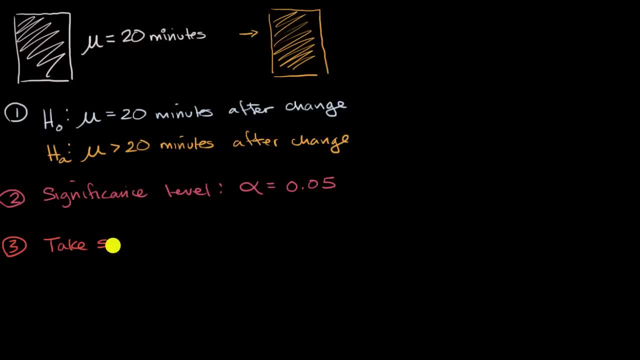 In step three we would take a sample, Take sample. So let's say we take a sample size. let's say we take 100 folks who visit the new website, the yellow background website, and we measure sample statistics. We measure the sample mean here. 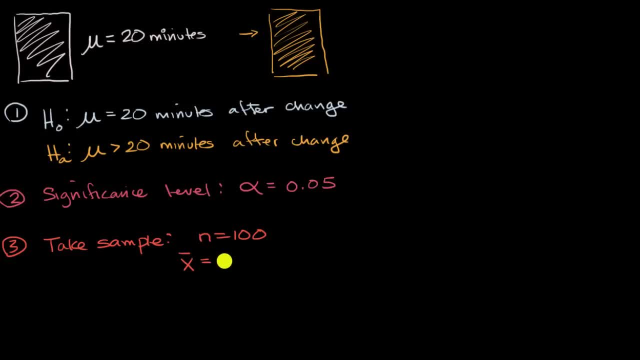 Let's say that the for that sample, the mean is 25, 25 minutes. We are also likely to. if we don't know what the actual population standard deviation is, which we typically don't know, we would also calculate the sample standard deviation. 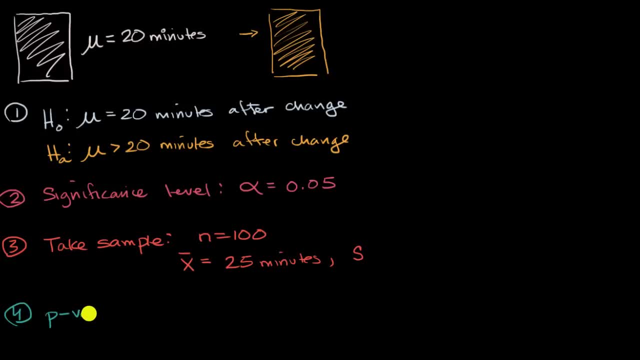 Then the next step is we calculate a p-value, And the p-value, which stands for probability value, is the probability of getting a statistic at least this far away from the mean, if we were to assume that the null hypothesis is true. So one way to think about it. 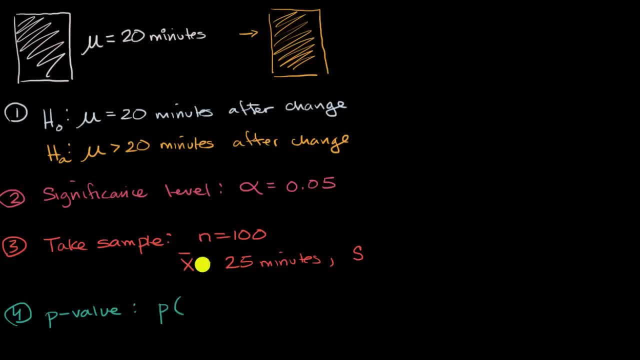 it is a conditional probability. It is the probability that our sample mean. our sample mean when we take a sample of size n equals 100, is greater than or equal to 25.5.. 25 minutes given, given our null hypothesis, is true. 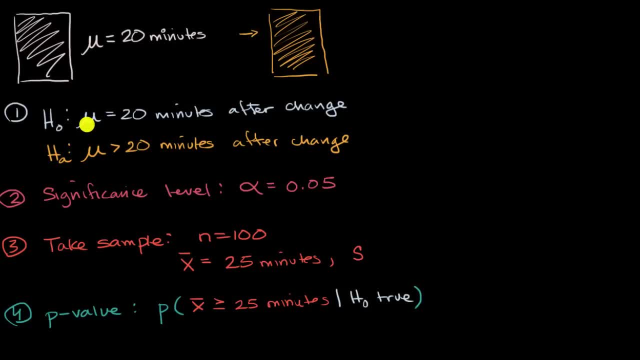 And in other videos we have talked about how to do this. If we assume that the sampling distribution of the sample means is roughly normal, we can use the sample mean, we can use our sample size, we can use our sample standard deviation. 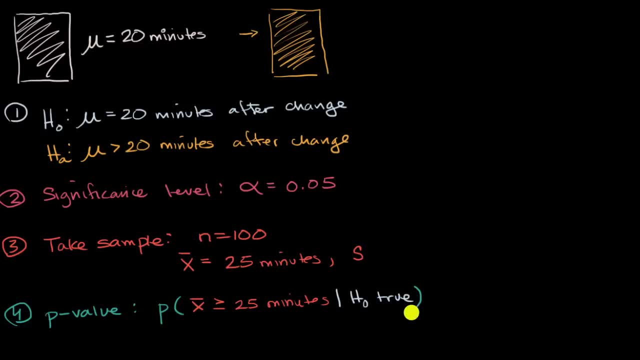 perhaps we use a t-statistic to figure out roughly what this probability is going to be, And then we decide whether we can do this, whether we can reject the null hypothesis. So let me call that step five. So step five, there are two situations. 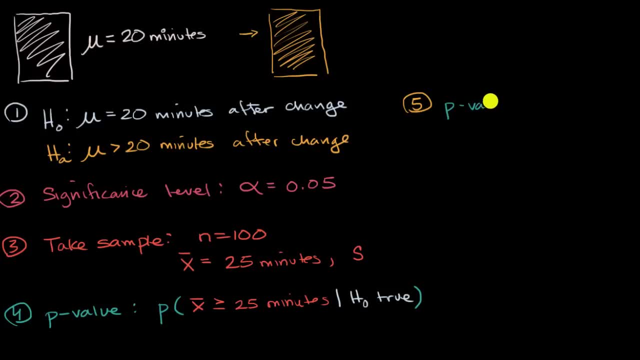 If my p-value, if my p-value, if it is less than alpha, then I reject my null hypothesis, Reject, reject my null hypothesis and say that I have evidence for my alternative hypothesis. Now, if we have the other situation, 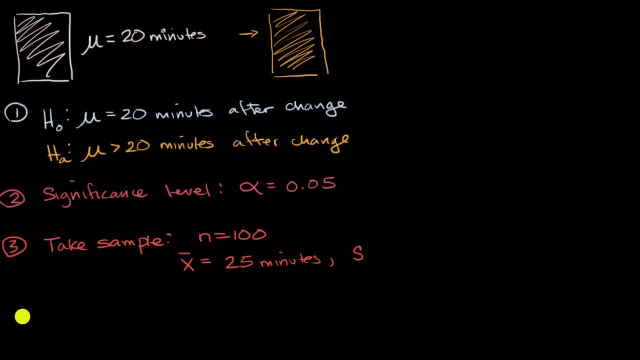 we would also calculate the sample standard deviation. Then the next step is: we calculate a p-value, and the p-value, which stands for probability value, is the probability of getting a statistic at least this far away from the mean, if we were to assume that the null hypothesis is true. 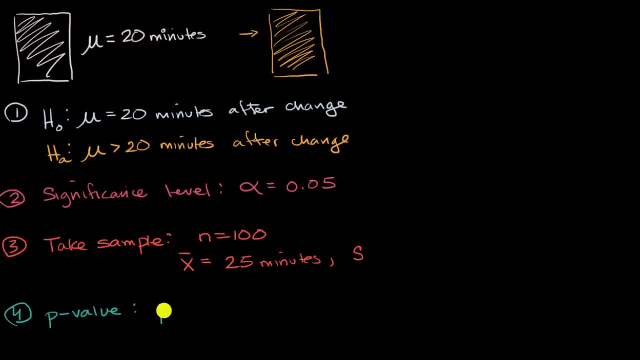 So one way to think about it, it is a conditional probability. It is the probability that our sample mean. our sample mean, when we take a sample of size n equals 100, is greater than or equal to 25,, 25 minutes. 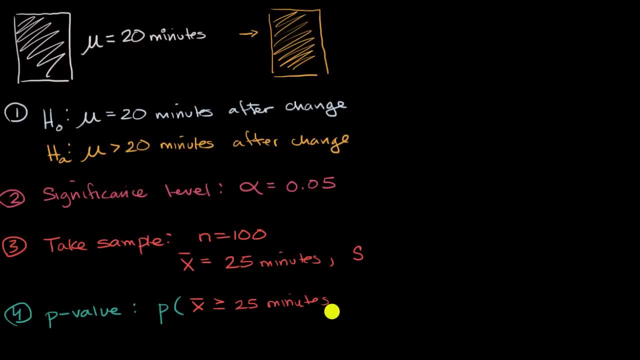 Given, given our null hypothesis is true, And in other videos we have talked about how to do this. If we assume that the sampling distribution of the sample means is roughly normal, we can use the sample mean, We can use our sample size. 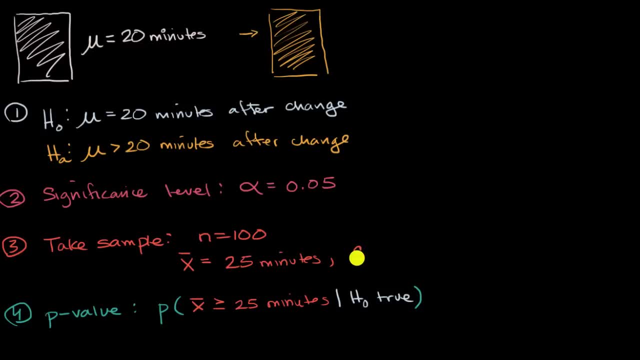 We can use our sample standard deviation, Perhaps we use a t-statistic to figure out roughly what this probability is going to be, And then we decide whether we can reject the null hypothesis. So let me call that step five. So step five. there are two situations. 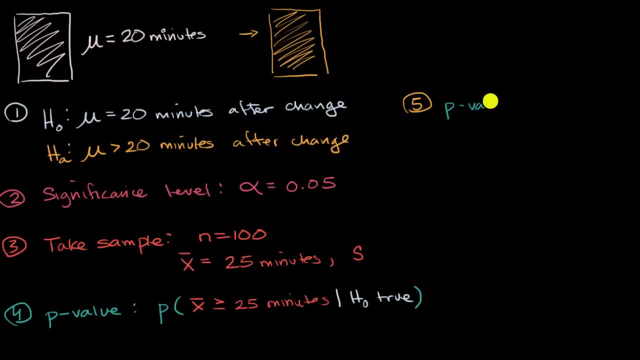 If my p-value, if my p-value, if it is less than alpha, then I reject my null hypothesis, Reject, reject my null hypothesis and say that I have evidence for my alternative hypothesis. Now, if we have the other situation, if my p-value is greater than or equal to, 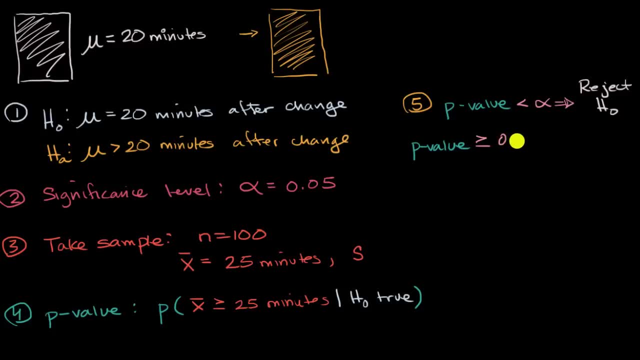 in this case 0.05.. So if it's greater than or equal to my significance level, then I cannot reject the null hypothesis. I wouldn't say that I accept the null hypothesis, I would just say that we do not do not reject. 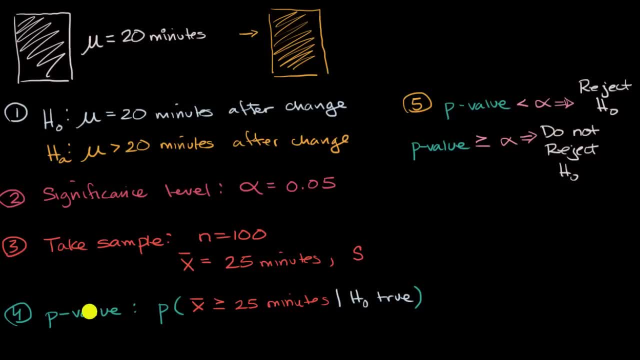 reject the null hypothesis. And so let's say, when I do all of these calculations, I get a p-value which would put me in this scenario right over here. Let's say that I get a p-value of 0.03.. 0.03 is indeed less than 0.05.. 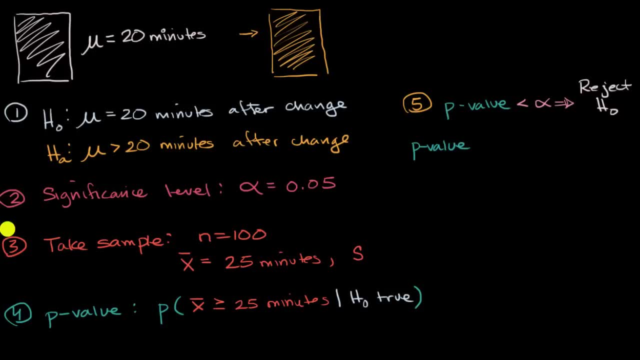 if my p-value is greater than or equal to- in this case, 0.05, so if it's greater than or equal to my significance level, then I cannot reject the null hypothesis. I wouldn't say that I accept the null hypothesis. 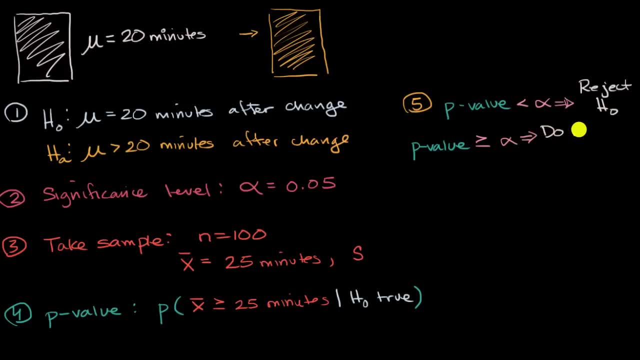 I would just say that we do not, do not reject, reject the null hypothesis. And so let's say, when I reject the null hypothesis, let's say, when I do all of these calculations, I get a p-value which would put me. 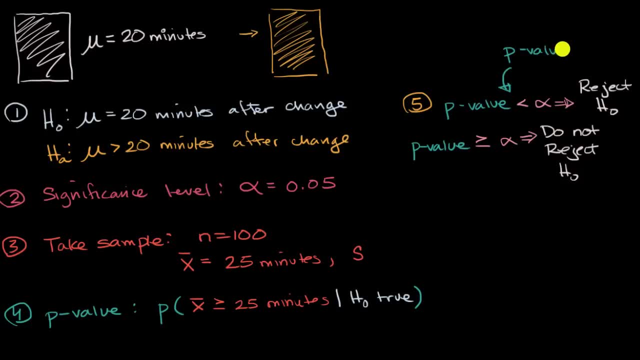 in this scenario, right over here, let's say that I get a p-value of 0.03.. 0.03 is indeed less than 0.05, so I would reject the null hypothesis and say that I have evidence for the alternative. 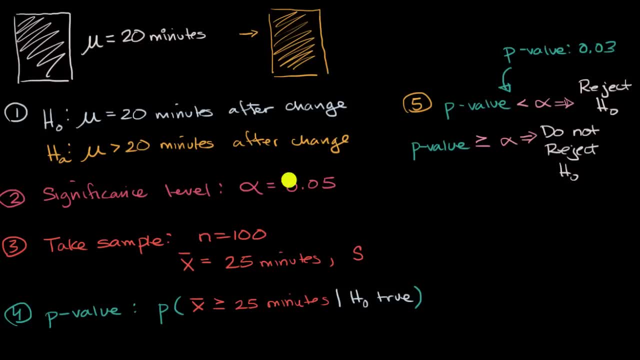 And this should hopefully make logical sense, because what we're saying is: hey look, we took a sample and if we assume the null hypothesis, the probability of getting that sample is three percent. it's three one-hundredths, and so, since that probability, 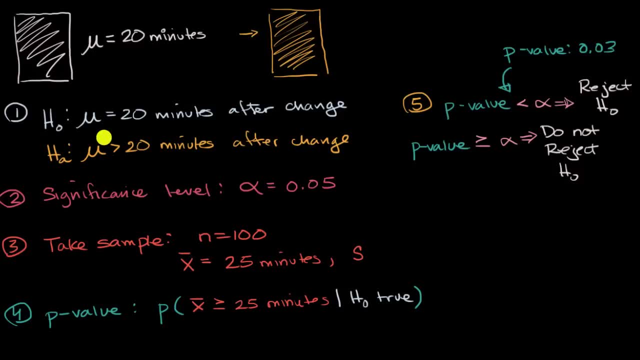 is less than our probability threshold here, we'll reject it and say we have evidence for the alternative. On the other hand, there might have been a scenario where we do all of the calculations here and we figure out a p-value, a p-value that we get. 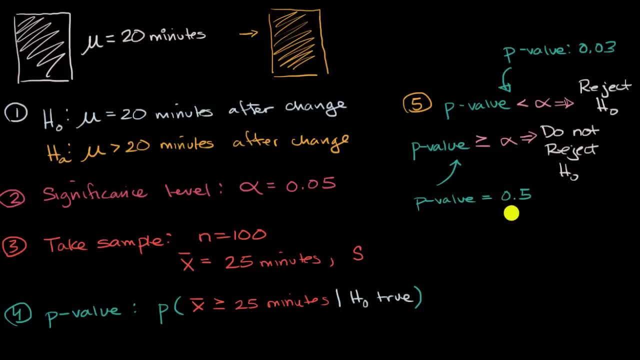 is equal to 0.5,, which you can interpret as saying that, hey, if we assume the null hypothesis 0.05,. which you can interpret as saying that, hey, if we assume the null hypothesis 0.05,. which you can interpret as saying that, hey, if we assume the null hypothesis is true. 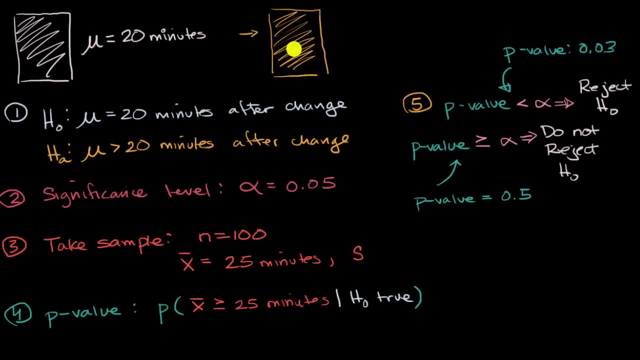 0.05, which you can interpret as saying that, hey, if we assume the null hypothesis is true, that there's no change due to changing making the background yellow, I would have a 50% chance of getting this result. 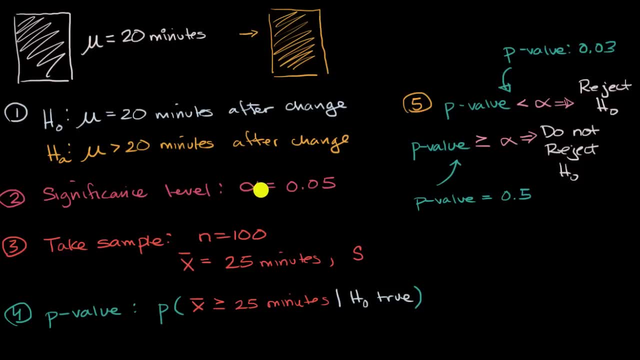 And in that situation, since it's higher than my significance level, I wouldn't reject the null hypothesis. A world where the null hypothesis is true and I get this result, well, you know, it seems reasonably likely, And so this is the basis for significant tests generally. 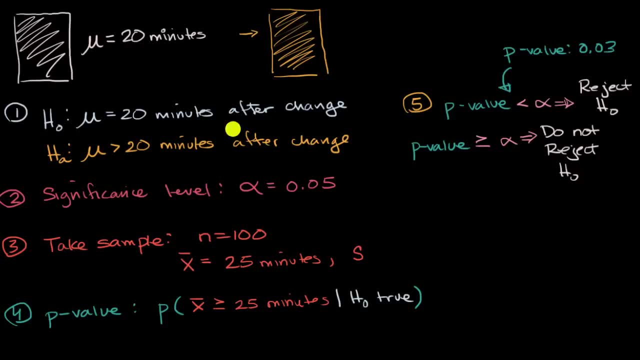 So I would reject the null hypothesis and say that I have evidence for the alternative, And this should hopefully make logical sense, Because what we're saying is: hey look, we took a sample and if we assume the null hypothesis, the probability of getting that sample is 3%. 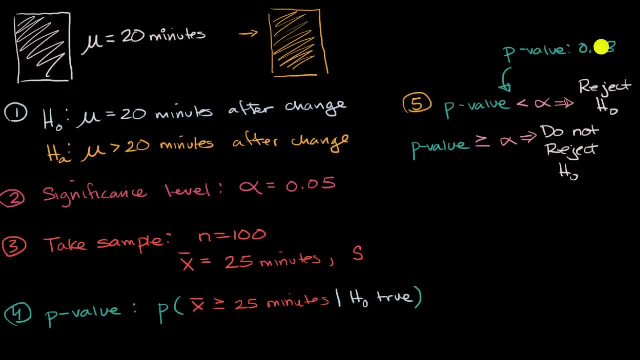 It's three one-hundredths, And so since that probability is less than our probability threshold here, we'll reject it and say we have evidence for the alternative. On the other hand, there might have been a scenario where we do all of the calculations here. 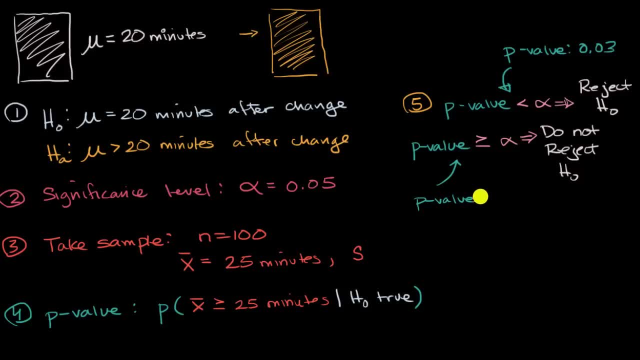 and we figure out a p-value. a p-value that we get is equal to 0.5.. Which you can interpret as saying that, hey, if we assume the null hypothesis is true, that there's no change due to changing, making the background yellow. 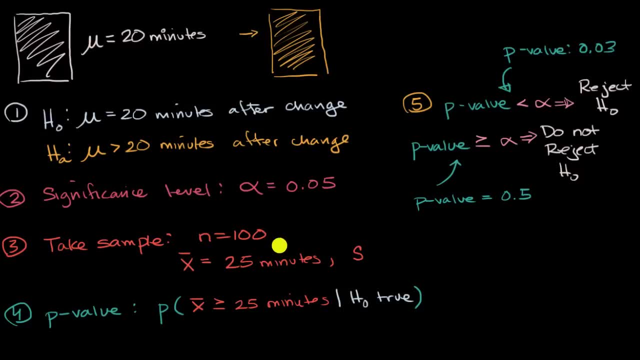 I would have a 50% chance of getting this result And in that situation, since it's higher than my significance level, I wouldn't reject the null hypothesis. A world where the null hypothesis is true, and I get this result. well, you know. 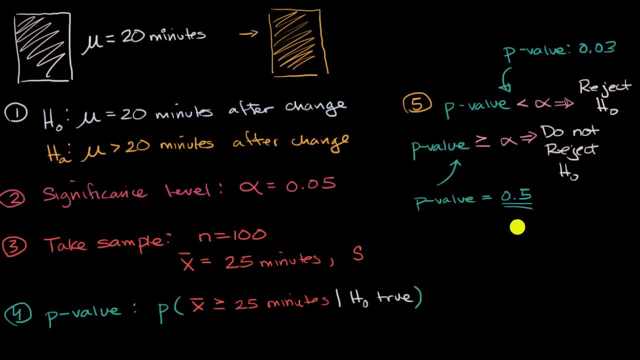 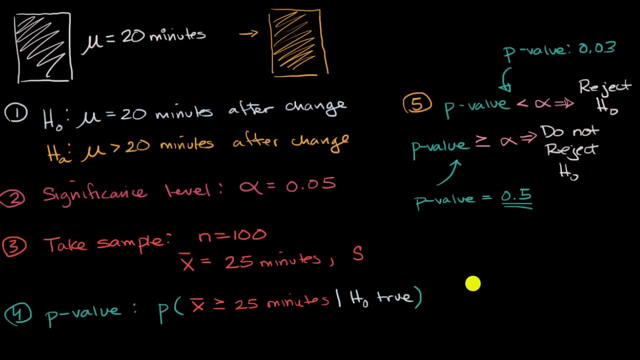 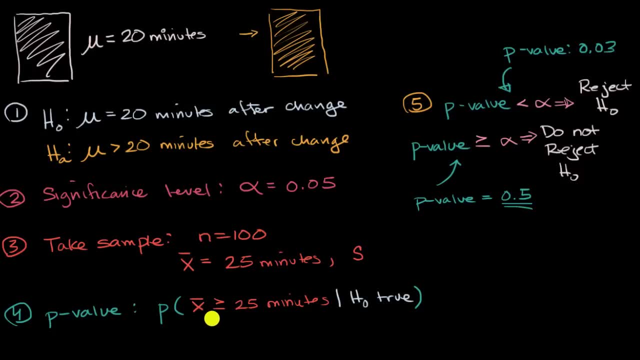 Our p-value, the thing that we're using to decide whether or not we reject the null hypothesis. This is the probability of getting your sample statistics, given that the null hypothesis is true. Sometimes people confuse this and they say, hey, is this the probability? 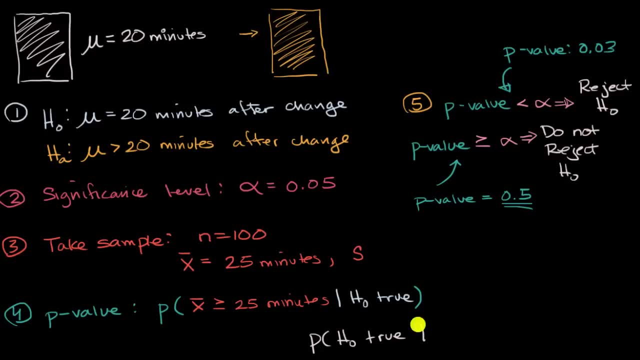 that the null hypothesis is true, given the sample that we got, and I would say clearly: no, that is not the case. We are not trying to gauge the probability that the null hypothesis is true or not. What we are trying to do is say: hey, 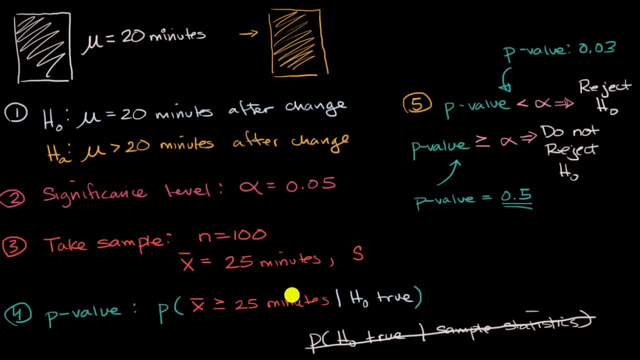 if we assume the null hypothesis were true, what is the probability that we got the result that we did for our sample? And if that probability is low, if it's below some threshold that we set ahead of time, then we decide to reject the null hypothesis. and say that we have evidence for the alternative.